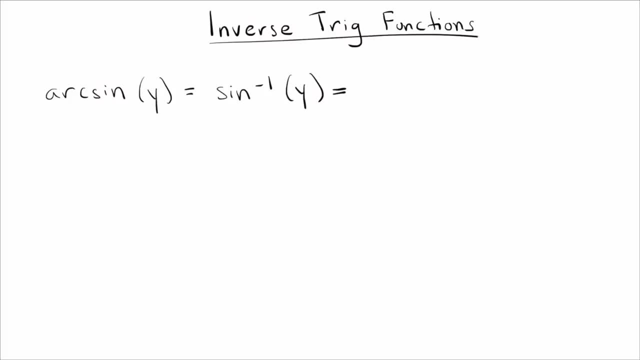 An important thing to note is: this does not mean the same thing as one over sine, and really the negative one means something a little different here. but just to avoid confusion, I'm not going to write it with the negative one. I like to write the arc to make it very clear. So generally what 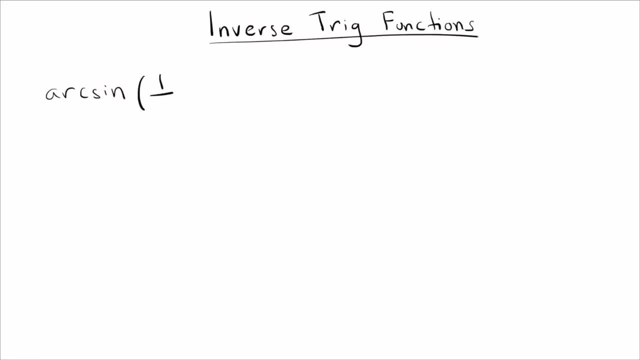 the questions will look like: is arc sine of something like maybe one over square root of two, and maybe they'll just ask you: what is this equal? or maybe they'll write something like equals x and ask you what x is. And of course, you can do the same thing for arc cosine, arc tangent, arc secant. 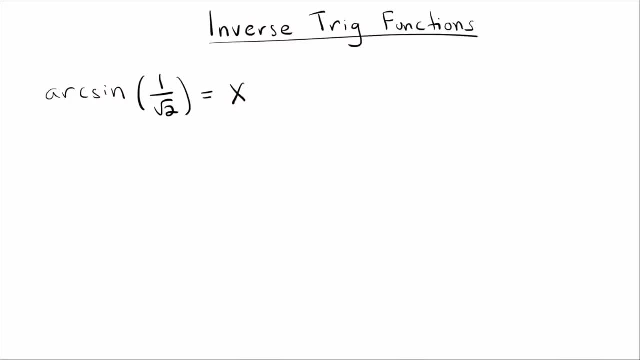 but let's just start simple with arc sine. So when someone writes something on the board or you see in a book that you don't know what that means, the first question you're going to ask is: what is this equal, or what is this equal, or what is this equal or what is this? 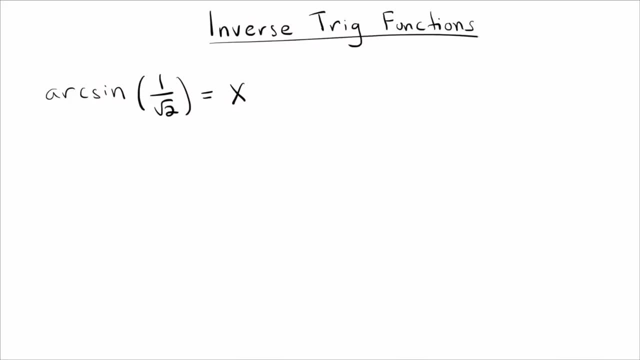 you should ask is: just what does this mean? I mean, just because someone wrote this word on the board doesn't mean you understand what it's actually trying to represent. So what does it mean? Well, if we write arc, sine of one over root, two equals x, what this means is simple. It means sine of what. 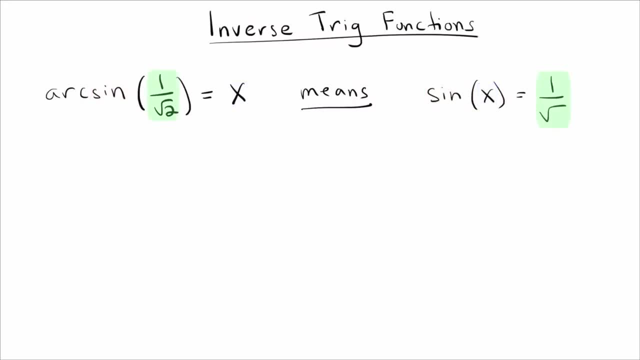 equals one over the square root of two. That's it. So these two things mean exactly the same thing, So you don't need to think of it as any fancy arc thing. It's just saying sine of what is one over square root of two. Okay so. 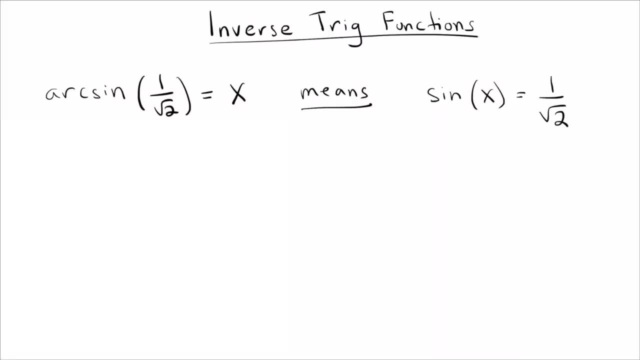 let's go ahead and work on what sine of what is one over square root of two? What angle do we need to plug in to get one over square root of two? So the first thing is we want to figure out where is sine going to be positive at, because this is positive, one over square root of two. So you may. 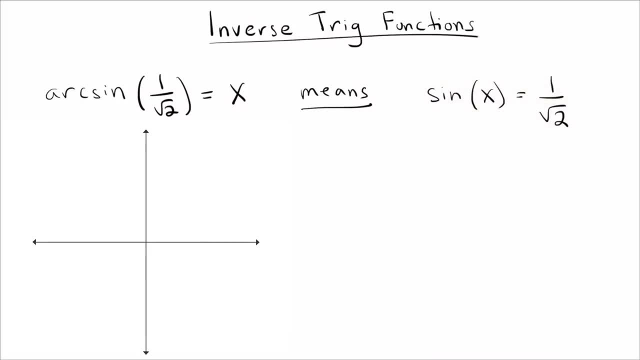 have learned this from different ways, maybe like an all students take calculus thing or something like this. But sine of what is one over square root of two is one over square root of two. So you can see that sine is positive in the first quadrant and in the second quadrant. So it could be that x. 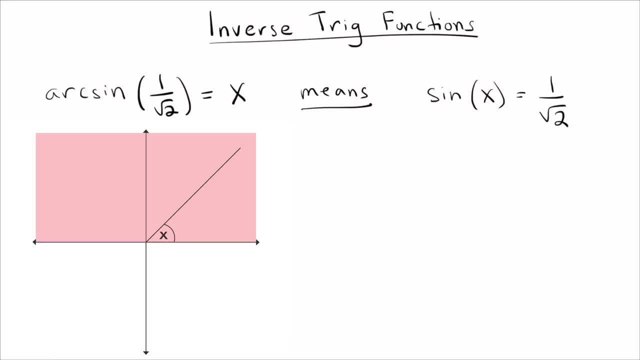 is this angle right here? or it could be that x is this other angle all the way in the second quadrant here. Okay, so I want to figure out what is x like. what is the angle actually? Okay, so all we do is very simple, right? What is sine? All that sine is is it is the opposite side divided by the 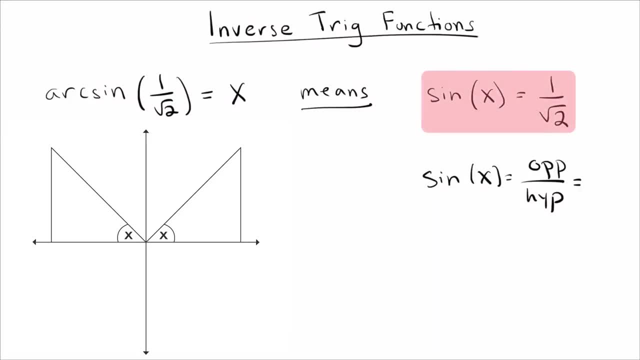 hypotenuse. So in our case, if we look above, we're going to have sine of what is one over square root of two. So the opposite side is going to be one for both of these and the hypotenuse is going to be square. 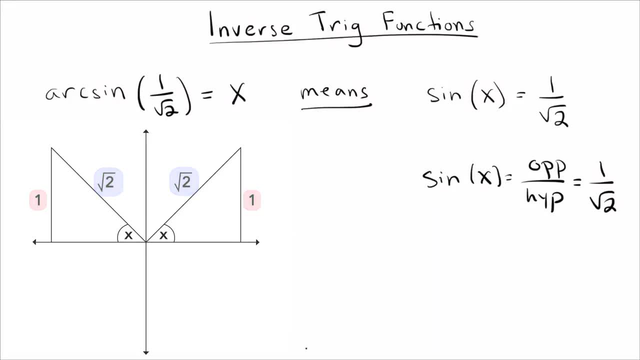 root of two for both of these. Okay, so all that's left now is to figure out this last side. You can use the Pythagorean theorem, or maybe you just recognize this triangle. but the last side is one, and over here it's negative one because we're going to the left, so that makes it be negative. 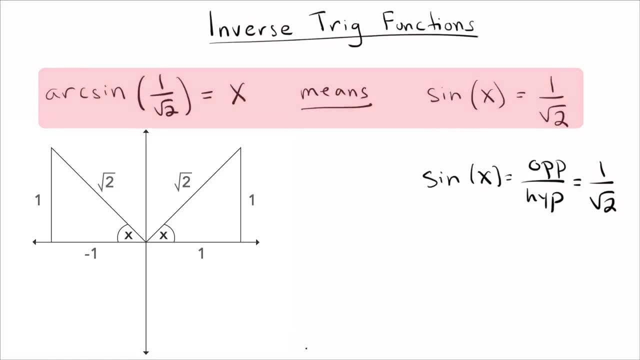 Okay, great. So our first step was writing out what does arc sine mean, And then we were going to mean: Our second step then was finding where could sine equal positive 1 over square root of 2, and then filling in our triangle. So nothing advanced yet, Okay. so the next thing now is: 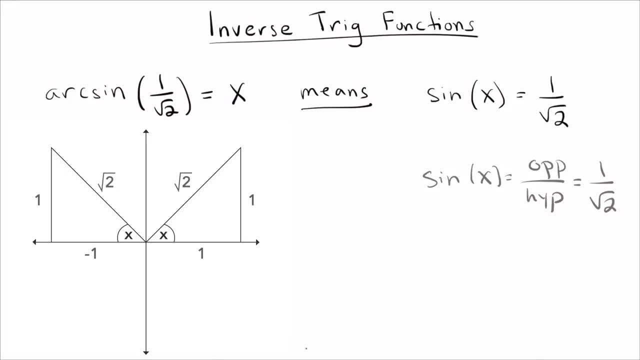 identifying what angle is x. And the way you do this is with your two special triangles. Remember, you've got the two special triangles. So your two triangles are the 45-45-90 triangle and the 30-60-90 triangle. In the 45-45-90, the sides are 1,, 1, and square root of 2.. And in the 30-60-90, they are 1,. 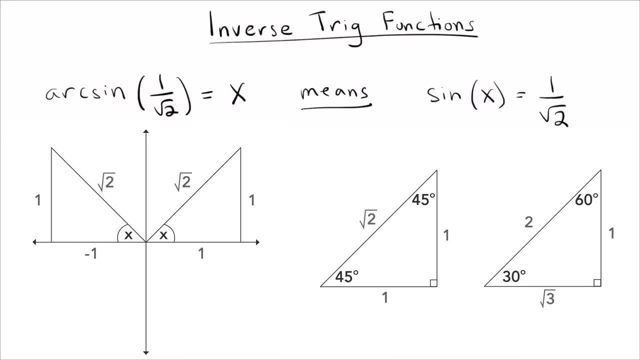 2, square root of 3.. So maybe you know this another way. Maybe you just memorized unit circle. That's fine. I'm going to go ahead and think about it from the special triangle way. Okay, so now we want to match it up. Okay, 1, 1, square root of 2.. Okay, I know what triangle that is. That is the. 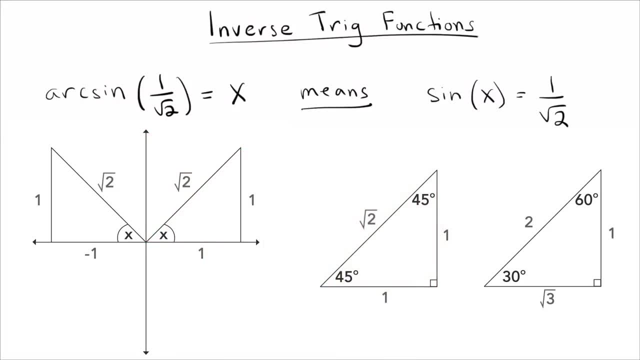 45-45-90 triangle. Okay, so I can just match it up and see that x is 45-45-90.. 45 degrees. Now I've done my work. You know what is x. We can see that for this first quadrant. 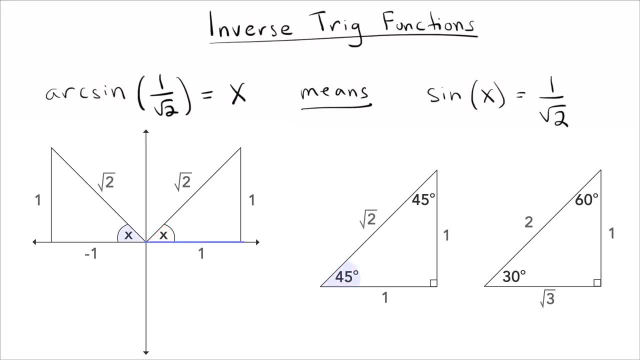 there x is 45 degrees. For the second one, the way I like to think about it is: you spin 180 degrees and you back off 45 degrees. So if I spun 180 degrees and I backed off 45 degrees, that would. 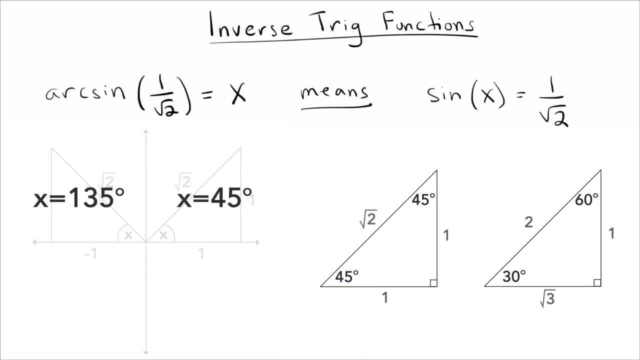 be 135 degrees. So I've got my two answers: x equals 45 degrees and x equals 135 degrees. But there's a little problem, And the problem comes from this word right up top here: functions. And what it is is that a function? all that means is if I plug in one number like, say, 1 over square, 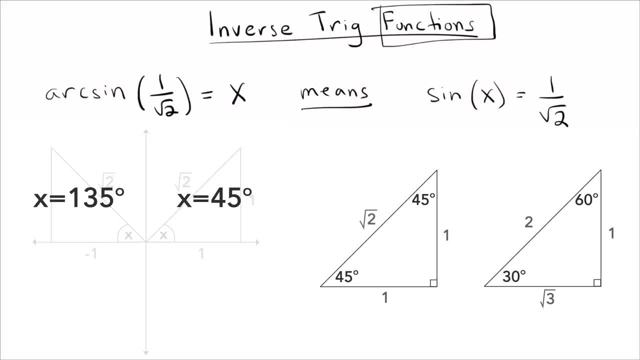 root of 2, I should get out one number. Plug in one thing, get out one thing. Well, I plugged in one number, 1 over square root of 2, but I got out two answers: 45 degrees and 135 degrees. 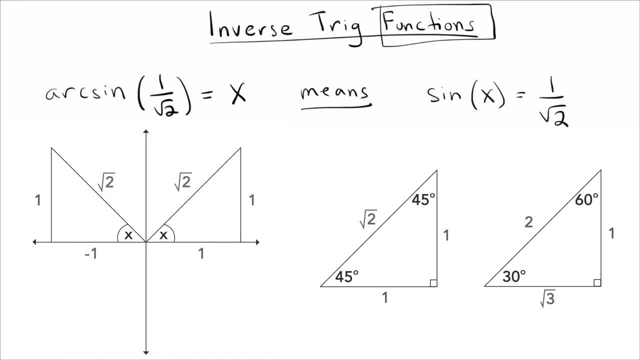 And in fact, if you're quick, maybe you'll notice that I actually got out two answers. I got out infinitely many answers. After all. there's no reason I have to just go 45 degrees. I could spin 360 degrees and then go another 45 degrees and I would get another answer of 360. 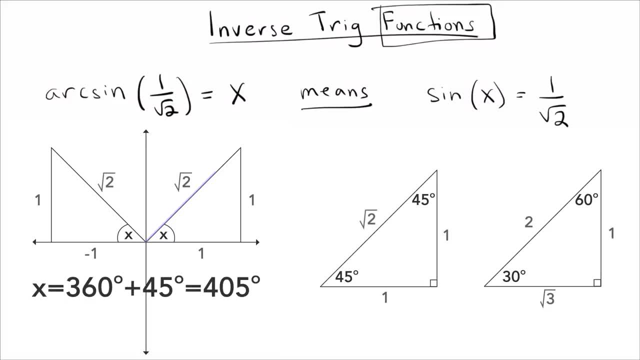 plus 45 is 405 degrees. And you could keep going forever and ever and you would get infinitely many answers. And for all of these answers, if you drew that angle and you took sine of it, you would get 1 over square root of 2.. So they're all. 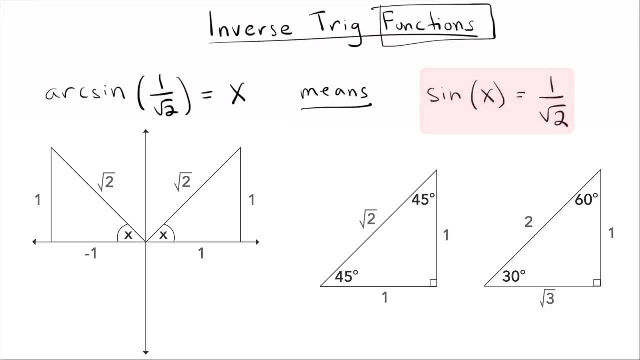 correct. they all give me 1 over square root of 2, but I don't want infinitely many answers. I want to get one answer so that if I do this problem and my friend does this problem, we get the same answer every time. Okay, so how do we fix that problem? Really, it's really simple, All you're. 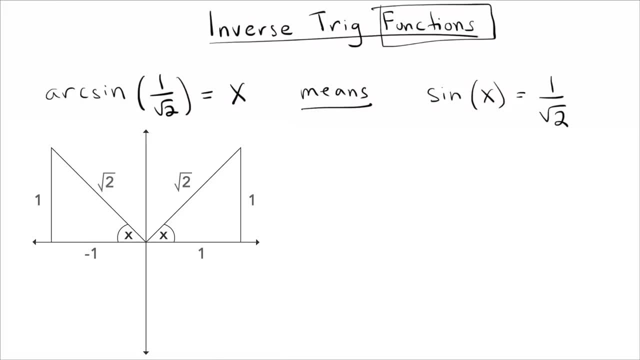 doing is adding one little extra condition. So let's write that out now. So if you open up any textbook that has trig in it, you're going to see a table that looks like this. It says: arc sine of y equals x means exactly what I just wrote. 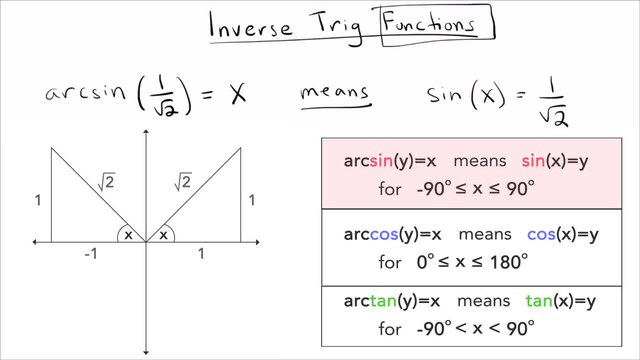 Sine of x equals y. So exactly the same thing as what I just did, But it's going to have one little extra condition on it. It's going to say for x between negative 90 degrees and positive 90 degrees, Or if you want to think about this in terms of radians, this is from negative pi over 2 up to. 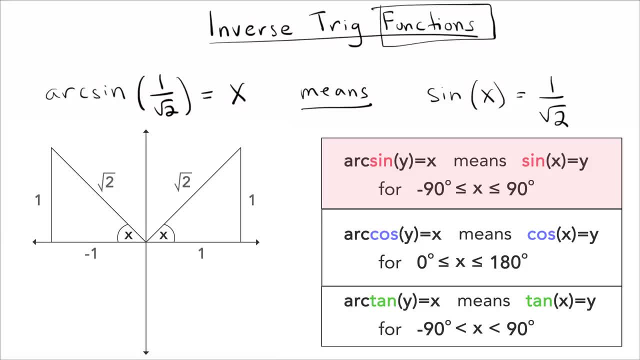 positive pi over 2.. So what is this saying? All this is saying is that the answer you get for x better be between negative and positive 90 degrees. So if you want to think about this in terms of x being negative 90 degrees and positive 90 degrees, those are the only answers we want. 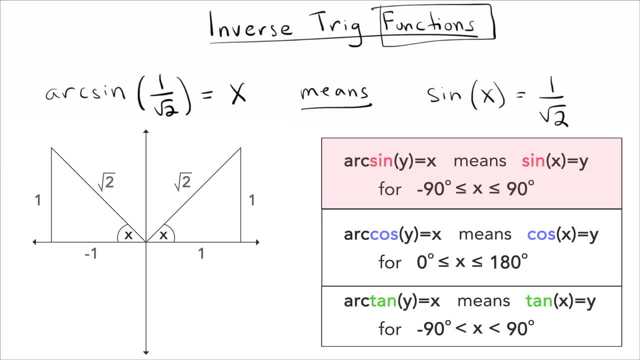 Anything that is not in that range we're throwing away, And by doing this, this forces us to have one answer for every single problem. So we saw before the different answers we got were x equals 45 degrees, X equals 135 degrees, And then we saw we could also keep spinning around, something like: 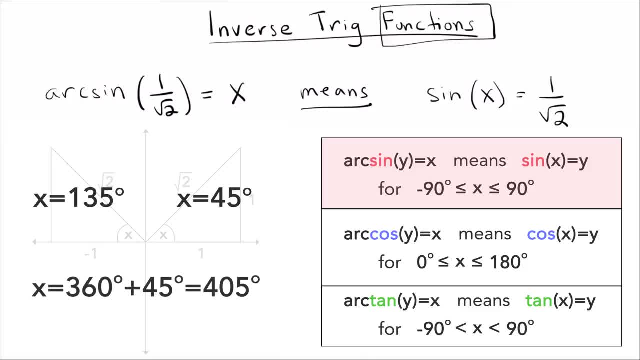 do 360 degrees plus an extra 45 degrees, and so on, And we saw that we could also keep spinning around something like do 360 degrees plus an extra 45 degrees, and so on, could keep playing this game, but what this does is it forces us to pick one. 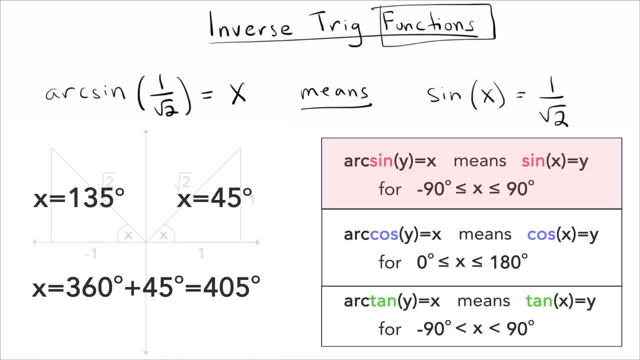 answer. I only want the answer where X is between negative 90 degrees and positive 90 degrees. this right here, 45 degrees, is the only answer that fits that. the rest of these do not match what my criteria says. so how can we save ourselves a little bit of time in the future rather than writing down a whole bunch of 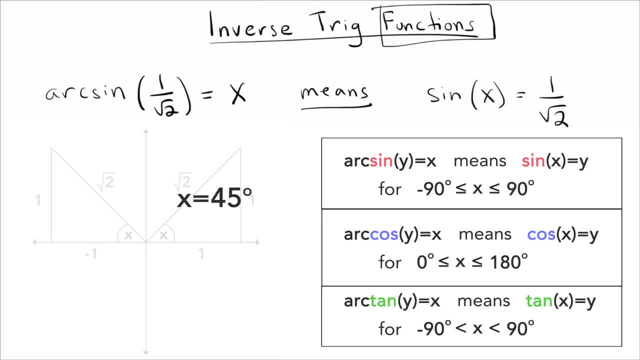 answers and then later going back and picking the one we want. all we need to do is just right, when we're drawing our special triangle, we can see which ones we want and which ones we don't want. so, for example, when we first draw our triangles here, we saw we had an X in the first quadrant and in the second. 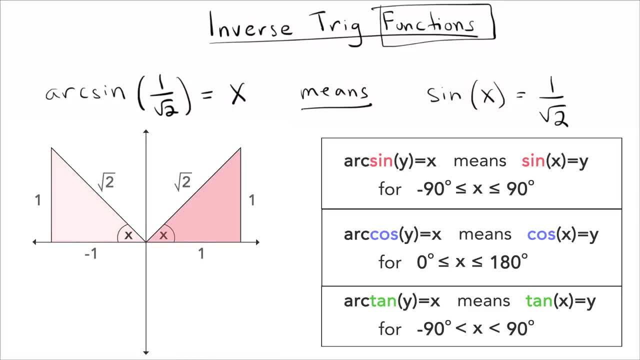 quadrant. well, if you think about an angle X in the first quadrant, that's between 0 degrees and 90 degrees. okay, that's good. 0 to 90, that is in the range I want. well, what about in the second quadrant? the second quadrant is between: 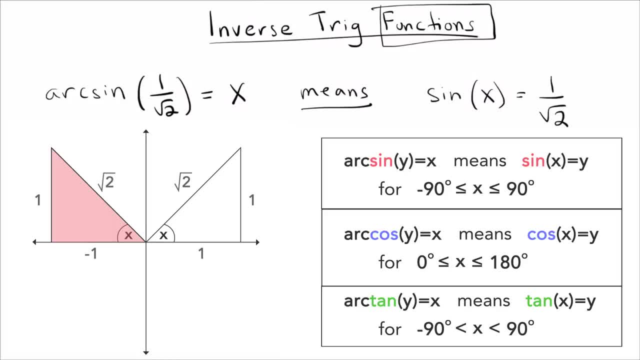 90 degrees, and 90 degrees and 180 degrees- that's too big right. I don't want things between 90 degrees and 180. it has to be smaller than 90 degrees. so right at the start I could have just thrown away that triangle. I didn't even need to deal with it. so that is how you. 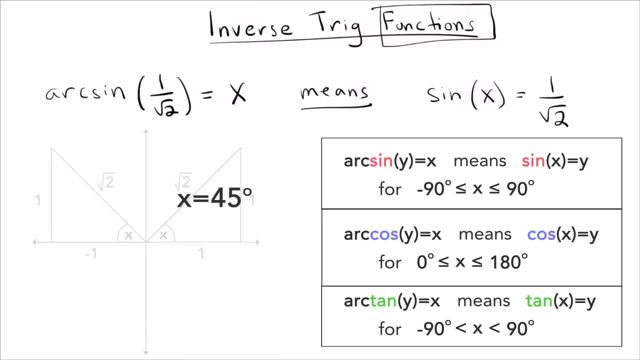 deal with these problems. so the final answer there is just: X equals 45 degrees, so that one probably felt long and you feel like man, these are a lot of work to do. they're really not. let's go ahead now and work through one together, that one's. 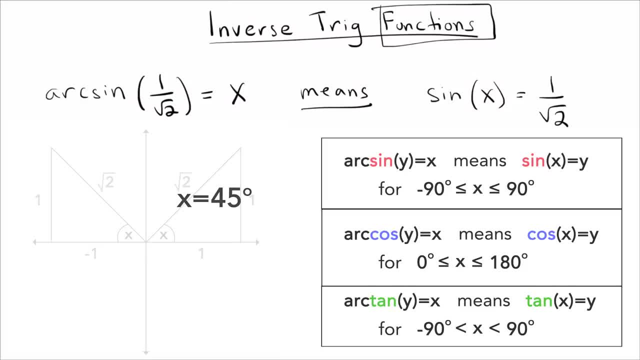 really not that bad. let's say you got a question like arc cosine of negative root, 3 over 2 and you're asked: what is this equal? sometimes the problems just say our cosine. I like to always write equals X and the reason I like that is: 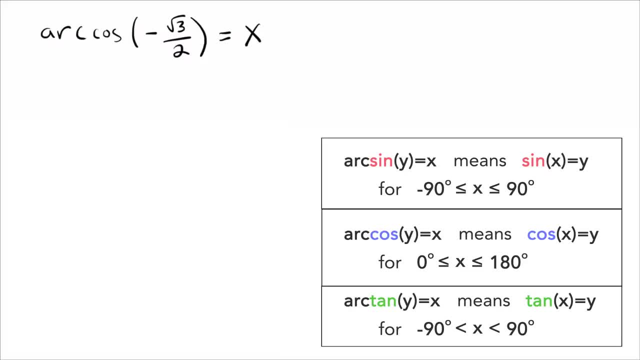 because then, at this next step, when I write out what this means- it's very easy to write out what it means. it means cosine of X equals negative 3 over 2. it's very easy to write out what it means. it means cosine of X equals negative 3 over 2. 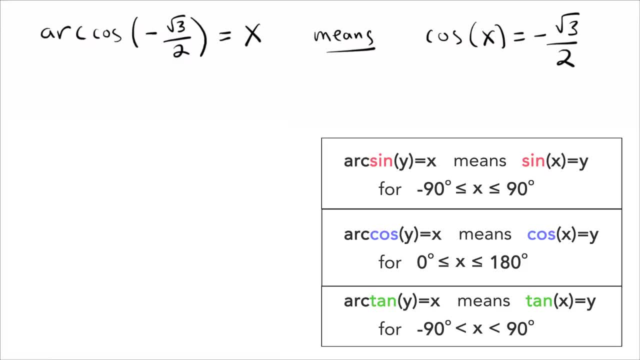 root 3 over 2.. Okay, so the first step was to figure out now where is cosine going to be negative at. So let's go ahead. We've got our axes here. So cosine is negative on the left, so up in the second quadrant and down in the third quadrant. Okay. so before we go any further, 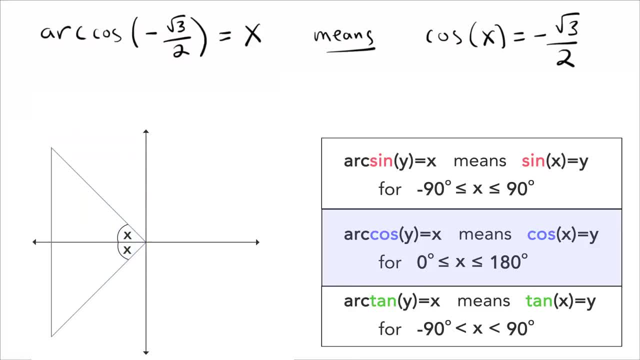 I want to think about my chart. So I already wrote a minute ago what the chart looked like for sine. For cosine, we see that x needs to be between 0 degrees and 180 degrees. Which one of these two x's is between 0 and 180?? It's the top one. It's the one in the second quadrant, This third. 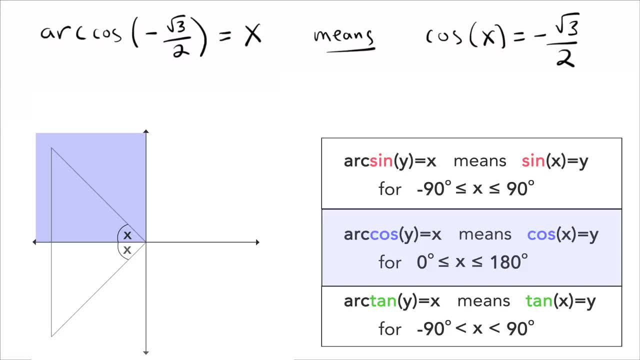 quadrant. it has to be bigger than 180 degrees, So that one I can throw away. Okay, so let's go ahead and finish the problem now. So we've got our triangle here. Cosine is adjacent over hypotenuse, So for us the adjacent side is negative root 3. The hypotenuse is 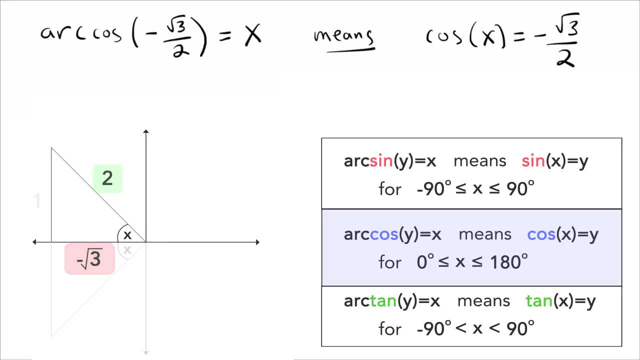 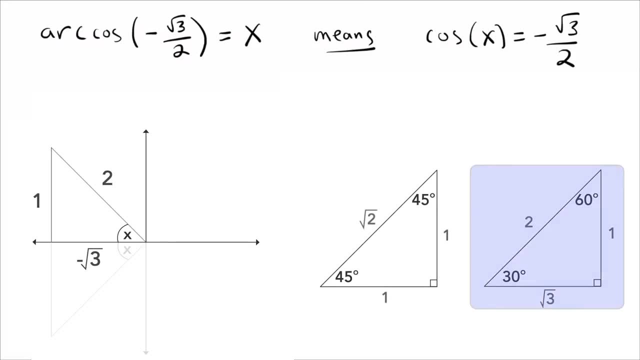 10. You go ahead and do your Pythagorean theorem. You find this last side is 1.. And you think about what is the 1,, 2,, root, 3 triangle, That is, the 30,, 60,, 90 triangle, And for that one, in fact, 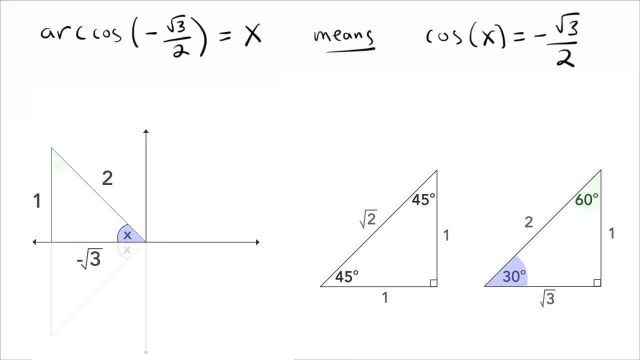 x is 30 degrees And the 60 degrees is up in this top corner here. Okay, so now all I need to do is write exactly how I get to this angle. How do I get right here? Well, again, I like to think of it. 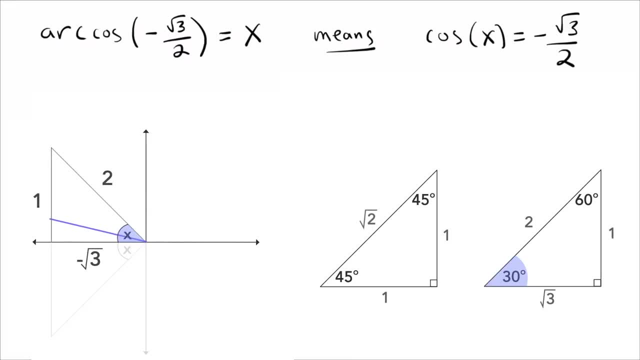 as I go forward 180 degrees and I back up 30 degrees, Which is the same as saying x is 150 degrees And there we go. We did the problem. So you can see, really there's not a whole lot of work involved in doing them. So I hope that helps, If you have. 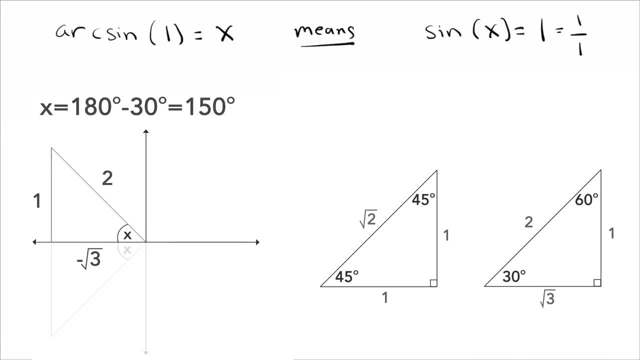 questions about these. you want me to do more of them? maybe a practice problems video? please let me know in the comments below and I'll be sure to get to that. Thanks everyone, and have a good one. Talk to you again soon.